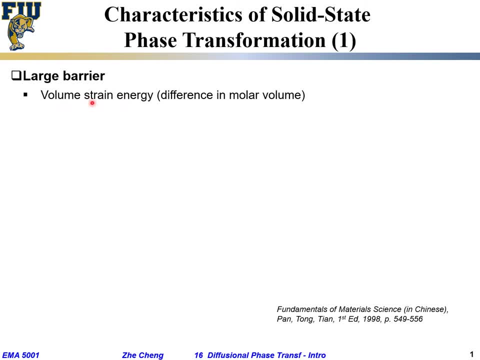 several aspects. One is the volume strain energy, which is due to the difference in the initial state and the final state in the molar volume. Quite often there's certain difference in the molar volume and to overcome the volume change and resulting strain energy. 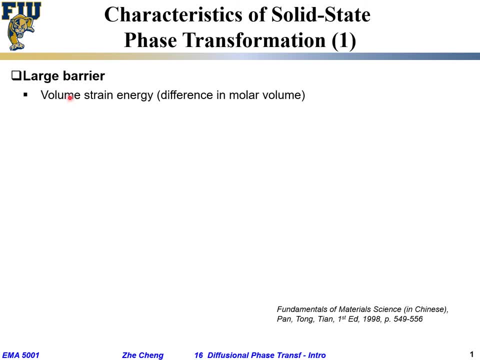 the volume needs a kinetic activation, and this is one part of the barrier where the resistance would come from. The other one is called interfacial energy, because between the different solid states there is quite often a distinct interface. and to create the interface 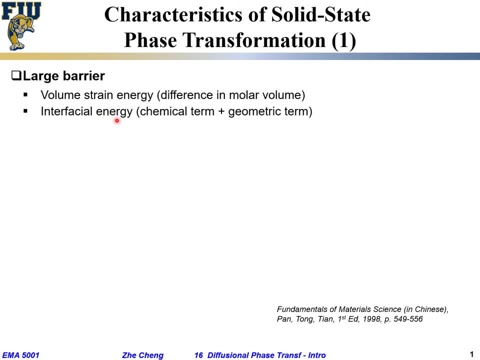 to realize the phase transformation from the initial state to final state. the interface creates the energy And the interfacial energy. as we mentioned before. it may come from different terms, such as chemical term. the interface atoms may be bonded to the run types of items which 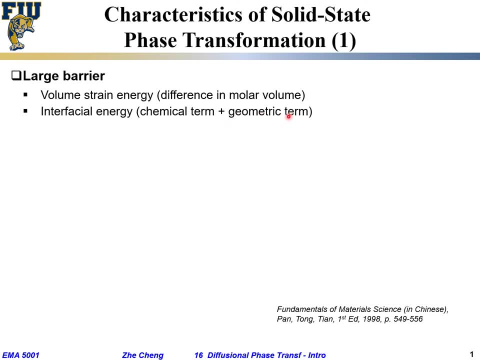 needs energy and also the geometric term. The new phase and the original phase may not match very well at the interface, and the geometry and the resulting strain energy will be very different from the previous phase. So this is one of the things that you need to be overcome. 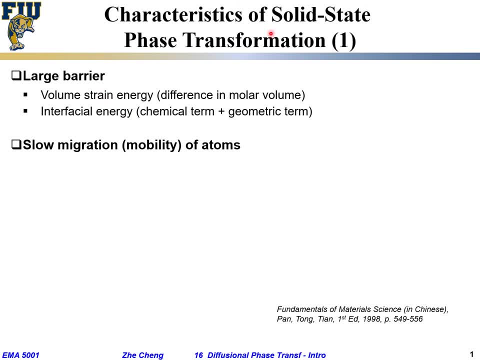 and this also constitute part of the barriers in the process And for solid state phase transformation. another characteristic is about the diffusion process or slow migration or low mobility of the atoms in the process. This is because atoms quite often are packed, they're pretty dense in the solid state. 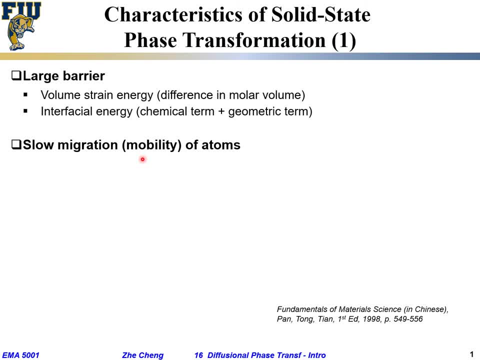 and the temperature is also lower. Therefore, in order for the atoms to move from one location to another location, it has to overcome the greater barrier. One example is about the self-diffusion coefficient in solid. The self-diffusion coefficient, which means even without concentration gradient for random work, the atom over time will. 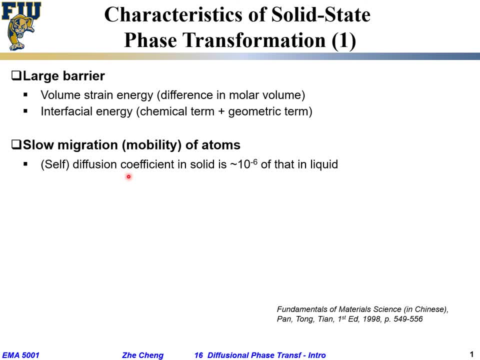 wander away from its original location. But the diffusion coefficient in solid, even without concentration gradient, is only one in a million of that in liquid, or 10 to the minus six of that in liquid, which means the diffusion in solid is much, much slower than in liquid. 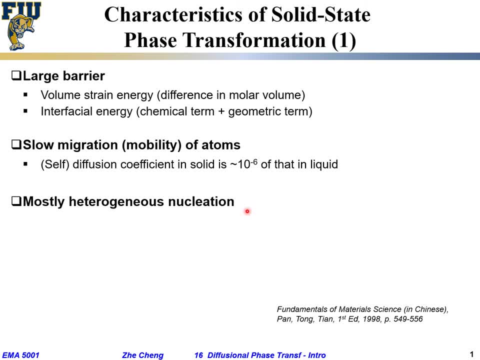 Okay, And because for solid state reaction, in most cases the phase transformation occurs through heterogeneous nucleation, which means the phase transformation process occurs at specific locations. that helps to lower the interfacial energy or reduce the stream energy. And this is due to the fact that all types of defects exist within the solid and they act as potential. 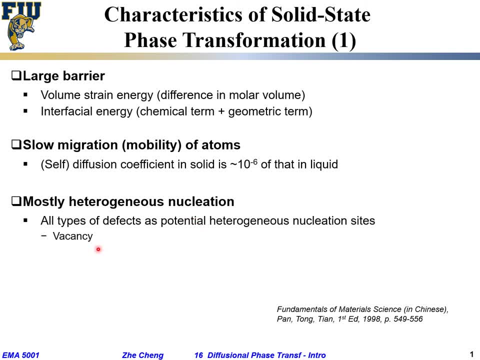 heterogeneous nucleation sites, For example. we talk about vacancies, that they can be and the vacancies are throughout the crystalline solid. There's also dislocation, a linear defect where the phase transformation would happen, Or green boundaries, that is quite often. 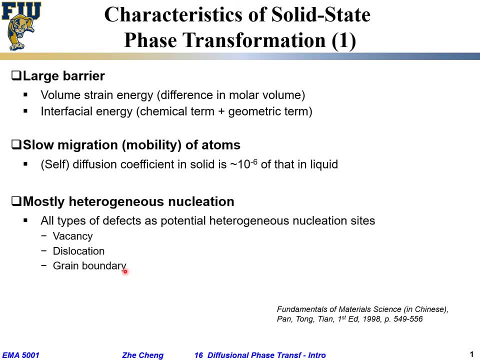 the location for many phase trans- solid state phase transformation to initiate because it's packed atoms are packed looser over there which can accommodate the stream energy And the interfacial energy And stacking forward can also be the location for phase transformation. Secondary phases which introduce extra interface will also be a 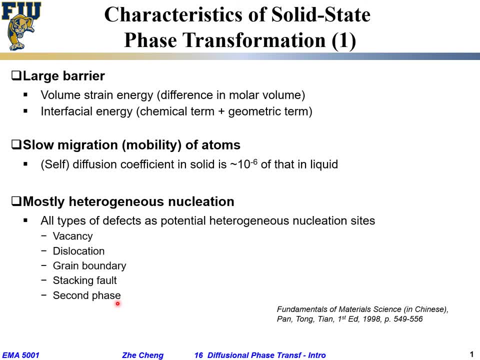 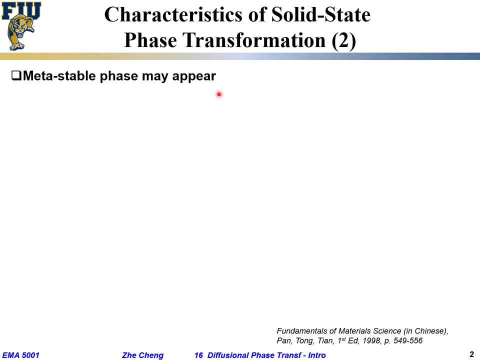 popular location for solid state phase transformation to initiate. Okay, And finally, of course, the material surface can also be a preferred location for heterogeneous phase transformation or nucleation sites. Okay, And in addition to the features that we mentioned, the slow diffusion. 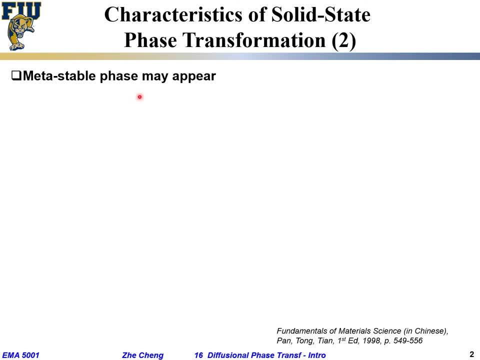 heterogeneous nucleation and large barrier. one other feature is that metastable phase may occur. When we say metastable state, these are the phase or state of material that is at a energy level that is higher than the ground state or the lowest energy state. 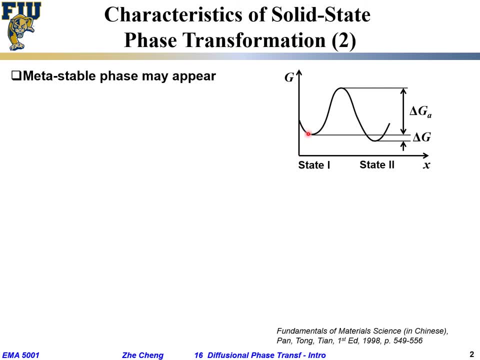 So here is a schematic which show a material that has two states, State one and state two, in terms of the Gibbs free energy, And what you see is that this state, too, is actually at a lower energy level compared with state one, But in between them there's a large barrier or large activation energy for the system to move from state one to state two. Thank you, So forане we now behave in a rotation, say at the beginiing state, then as a glулиkinization state, We can temporally add our two state elements in order to create a rotation state based on exchange power. 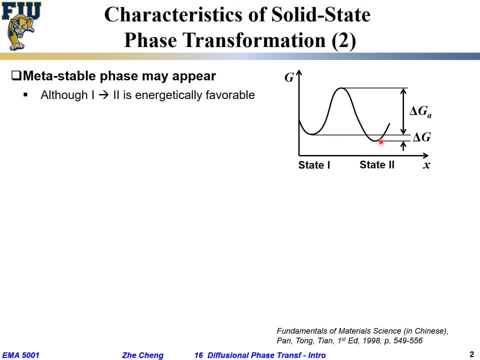 two. because of this large barrier, even though from state one to state two is energetically favorable, which means from state one to state two, the system actually gives free energy, decreases the process. sometimes do not readily happen because of the existence of large barriers. for example, as you will see here, from state one to state two, even though the free energy drops. 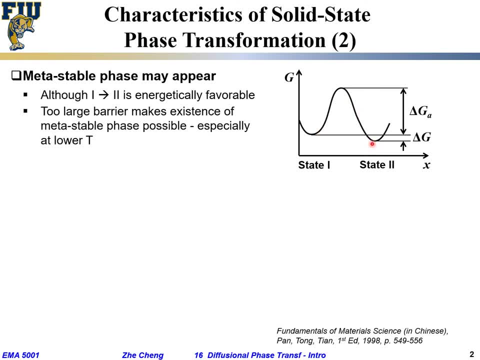 it has to overcome a steep energy barrier, or activation energy, in order for the transformation to occur from state one to state two and, as a result, the probability of that is low from one to two, and quite often the material would stay in the metastable state of state one instead of moving all the way to the most stable state of. 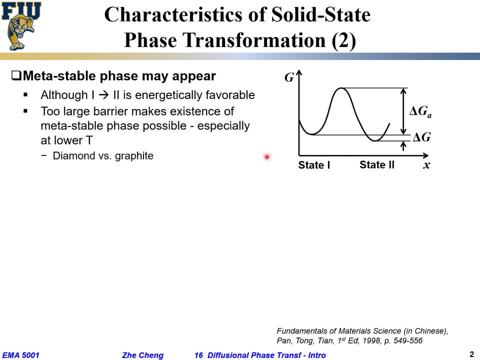 state two. okay. the one example would be the diamond versus graphite. we all know both diamond and graphite are pure carbon in terms of element composition, but on the other hand, people know that graphite is the most thermodynamically stable phase at ambient condition, at room temperature. however, 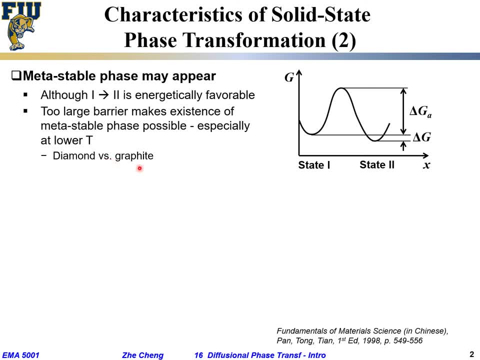 even though diamond is has an energy state that is somewhat higher than graphite at room temperature, diamond crystals do not readily transform into the lower energy graphite diamond do not transform to graphite at ambient condition. because why? because of this huge activation energy, because of slower diffusion. okay, and another example is about anolytese to tiO2 versus a rutile tiO2. 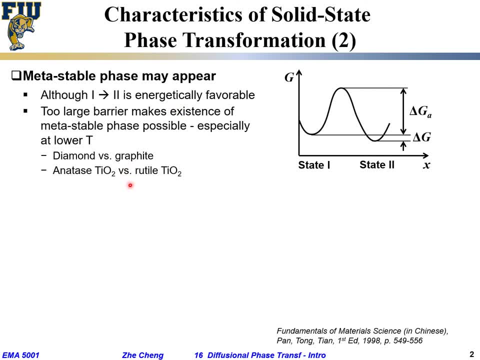 both these two types of tiO2 or titanium dioxide have the same metal of titanium and the same non-metal atoms of oxygen, and the ratio is one to two between titanium and oxygen. however, the anatase phase has a different crystal structure. it actually has three. 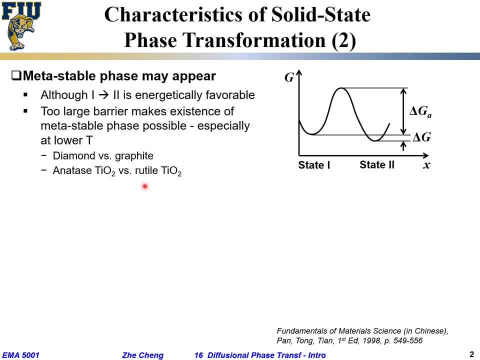 anti- равно events at negative underground Test. phase two is what i recall from my definition, and so is laboratories method. when I looked at both of them I found some from the rutile TiO2 phase, and actually the anatase phase would be of higher energy state. 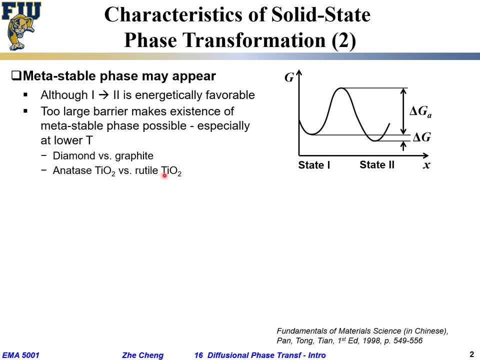 compared with TiO2 state, especially at comparable low temperatures. okay, but because of the large barriers between those two states, the produced anatase quite often stays as anatase unless you heat them up to to achieve the phase transformation. completely okay. and another feature is that 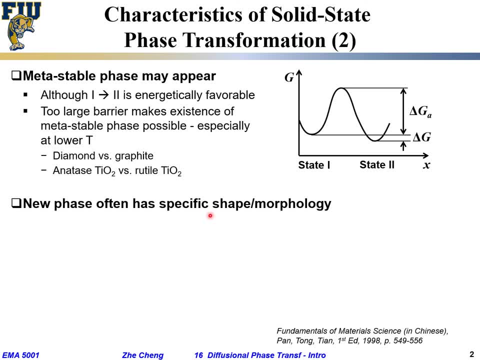 the new phase that are formed, often have specific shape, or we call morphology or appearance. okay, and for those that are interfacial energy controlled, which means the new phase and the old solid phase has a large interfacial energy. so then the process, the transformation from: 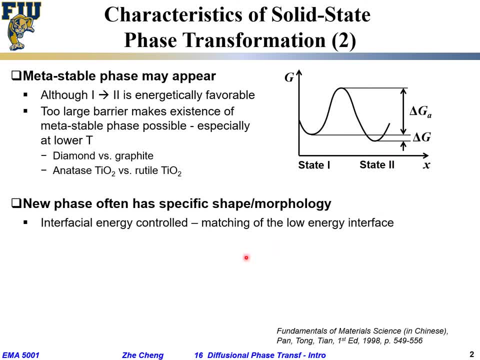 initial state to final state. quite often they try to match the lowest energy interface, lowest energy interface between the two phases, if they can find one. quite often the shape of the crystal is determined by how well it match between the initial state and the final state and how big a barrier. 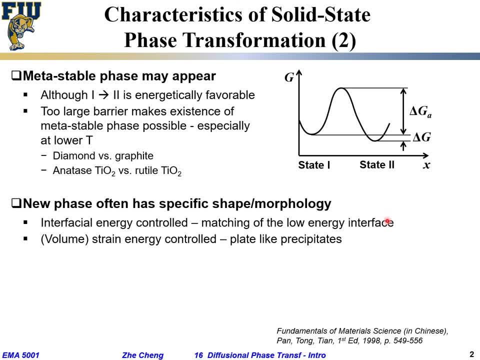 that exists between those two, okay. and for systems stream energy or the system gives free energy, as we mentioned before, quite often they form a precipitate in order to reduce the volume free energy and term in order to lower the system- free energy, okay. and the final feature about